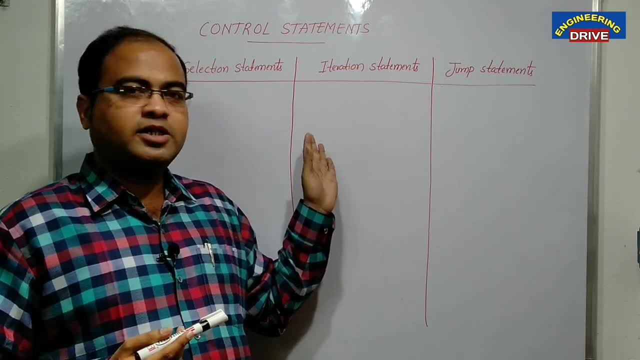 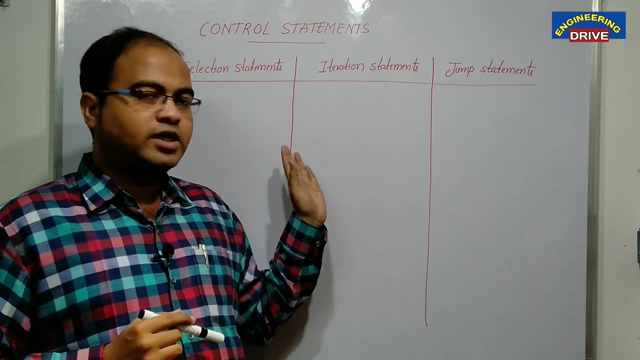 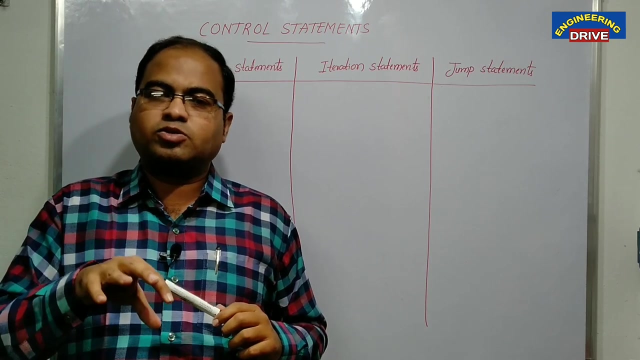 C++ or Java. these concepts will be used in most of the programming languages with slight modifications. So my goal is: I want to make sure that you know each and every topic in clear. Okay, whatever I am going to discuss, these concepts you can implement in all the 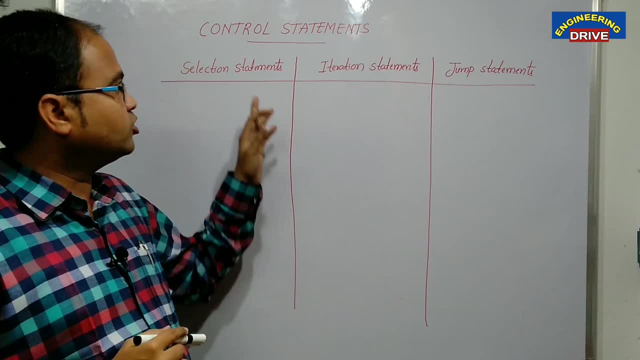 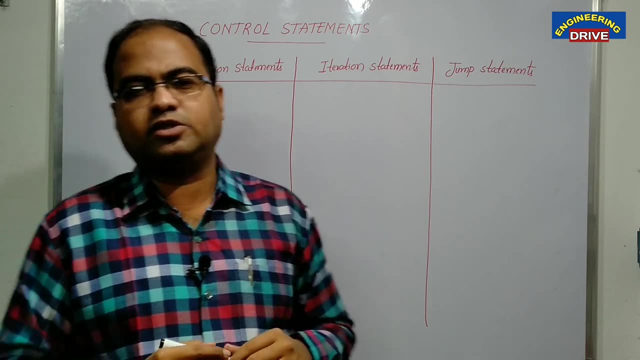 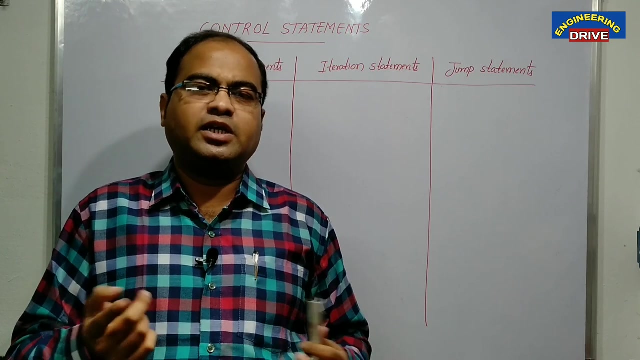 programming languages. So the name of the topic that I am going to discuss today is the control statements. Okay, what are the control statements supported by our C language? Even though I am discussing about C, if you compare the same topic in Java, 90% it will be. 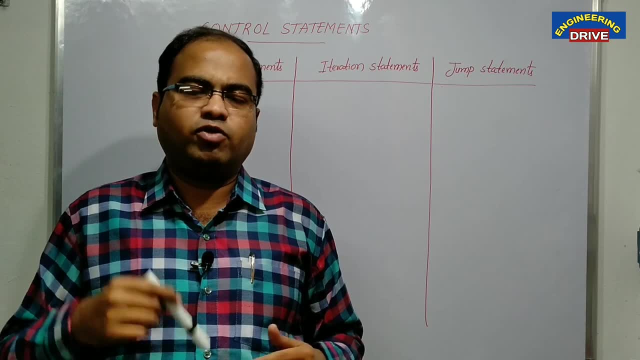 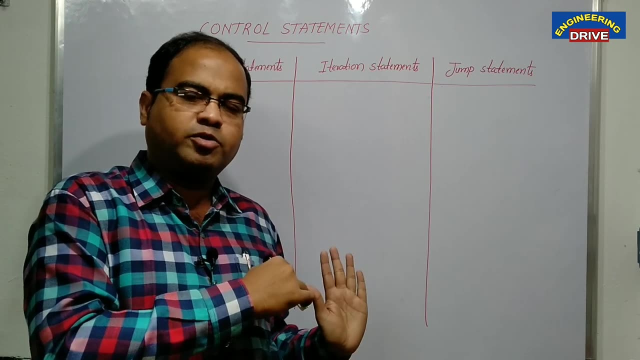 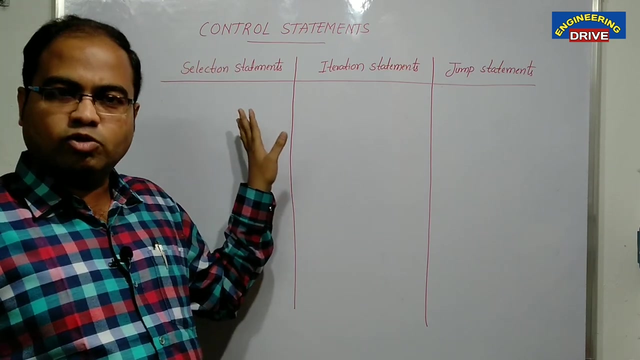 same with 10% modifications. Okay, and if you compare it with C++, also there will be slight modifications and you can know there is no harm that you can use the concept of C in other languages. So what are the different types of control statements supported by our C language? 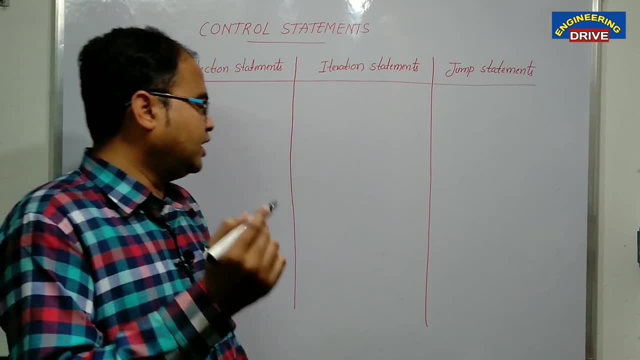 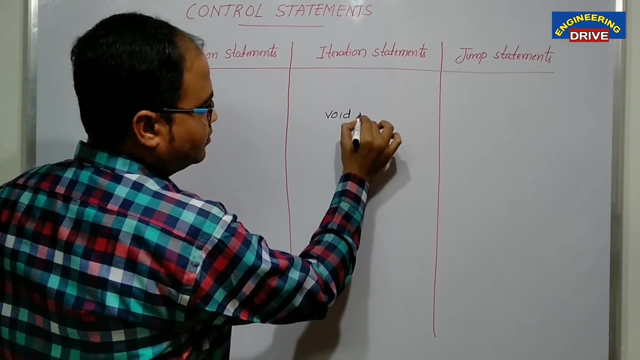 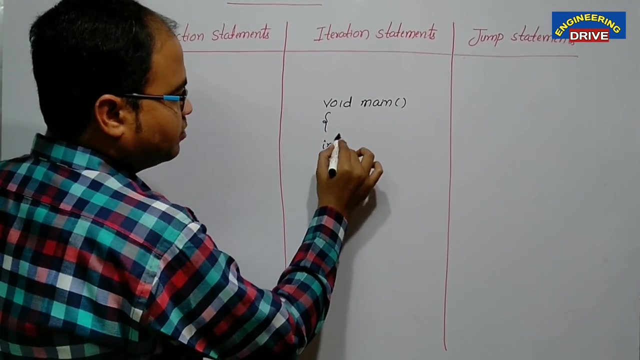 First of all, what is control statement? Control statement means generally how our C program will be executed from top to bottom. You will write, we will write our C program, Okay, and then we will write some statements. Suppose I want to display value of the variable CLR. 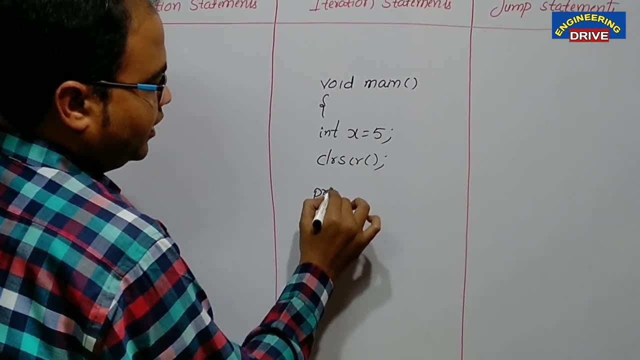 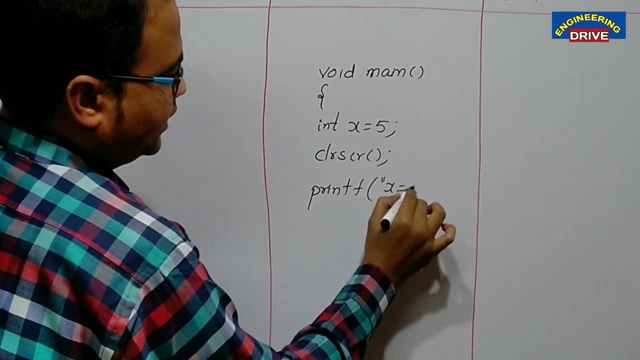 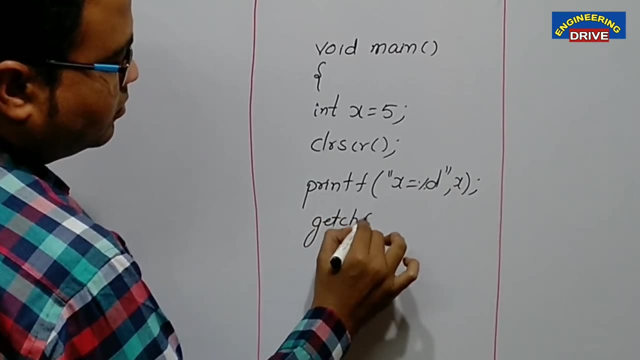 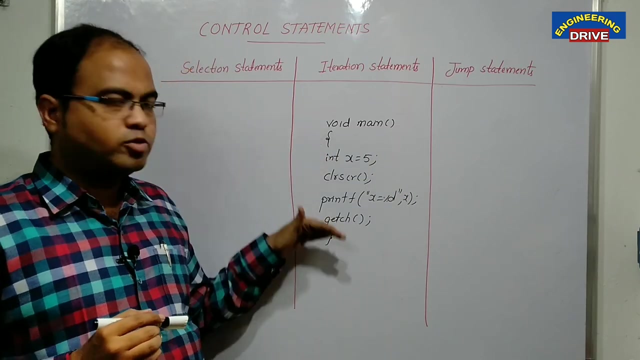 x is equal to %d, comma x. next getch program closed. Now how this program will be executed. This program will be executed always from top to bottom in sequential order. So it will start from suppose. if you write header files, it will consider the header files next wide. 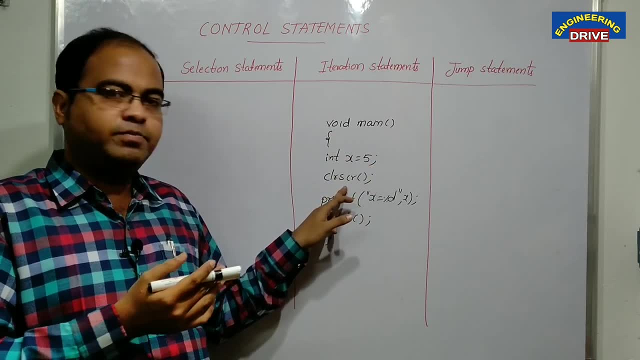 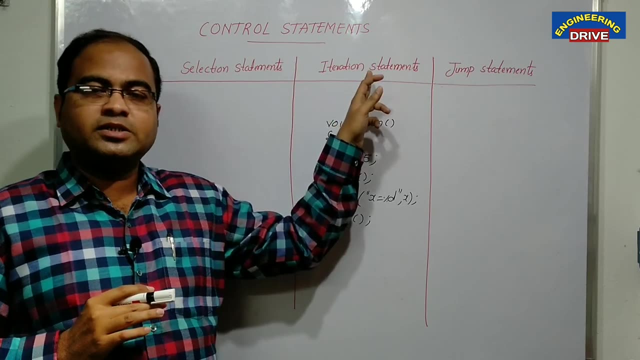 main opening brace. next value will be initialized, Then previous output is cleared In the. So the outcome will be: dah nah, nah, nah, no blocks, All this RANDOM stuff. Next, control displayed. output will be displayed and then program will end. sequential order control statement means: 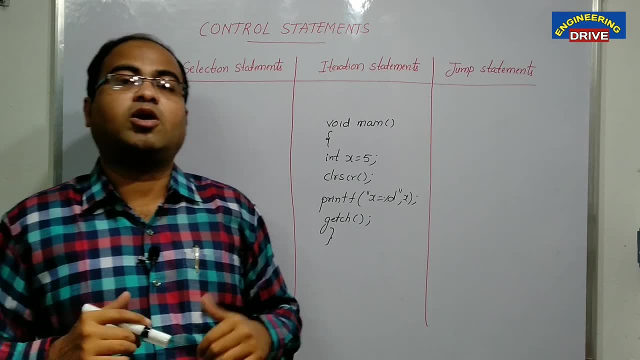 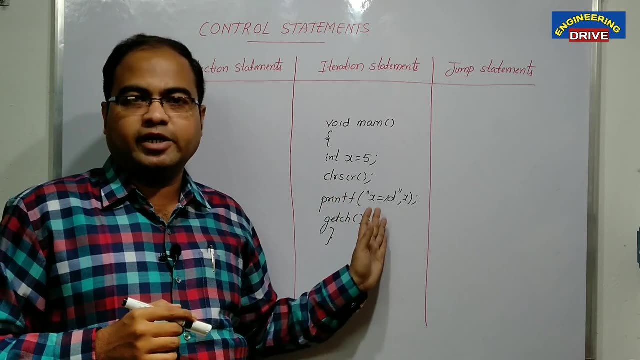 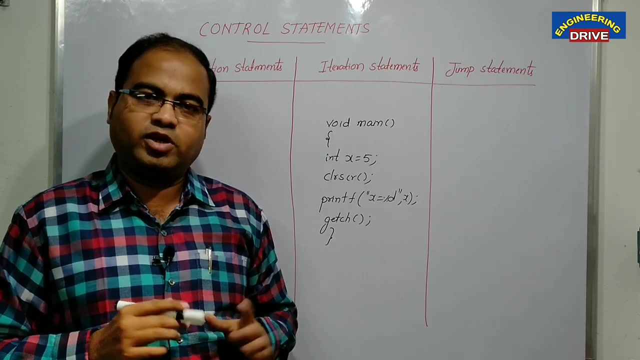 control statements is nothing, but sometimes i want to change the order of execution depending on some conditions. based on some condition, i want to execute my statements. then at that time we need to make use of this control statements, which is provided by our c language. okay, hope you got idea. generally, our c program executes in sequential order. if i want to change the order, 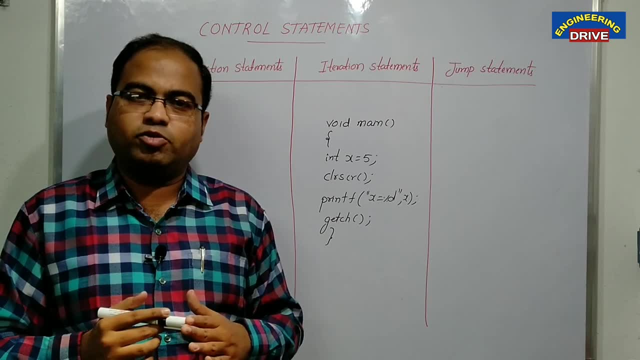 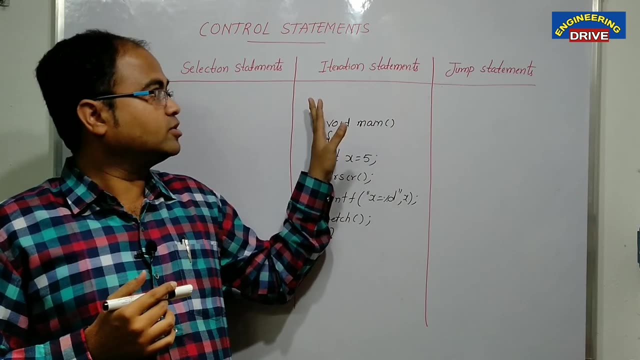 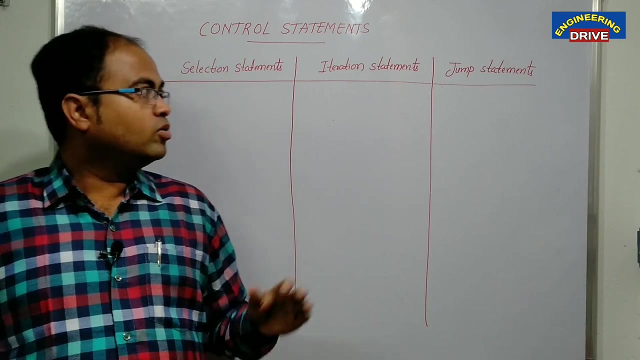 depending on some conditions, the statement must be executed. then c language provides a very important topic: that three types of control statements are available for us. okay, what are those? what are the different types of control statements we will see in our today's video? okay, so these are the three types of control statements supported by our c selection statements. 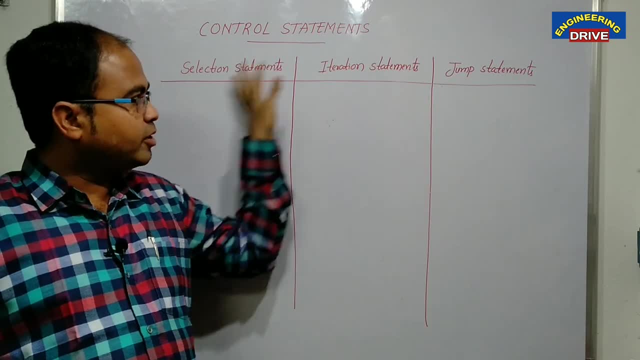 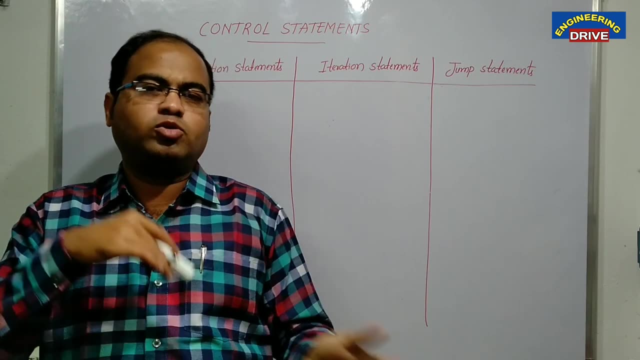 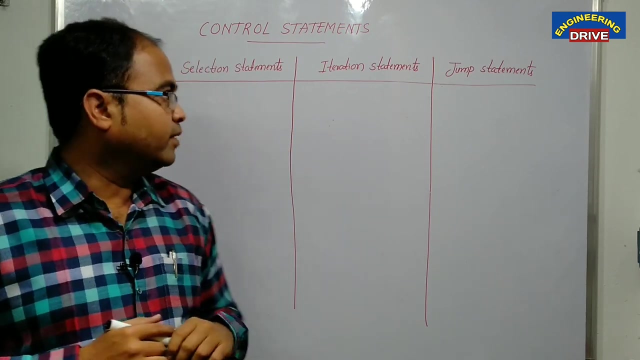 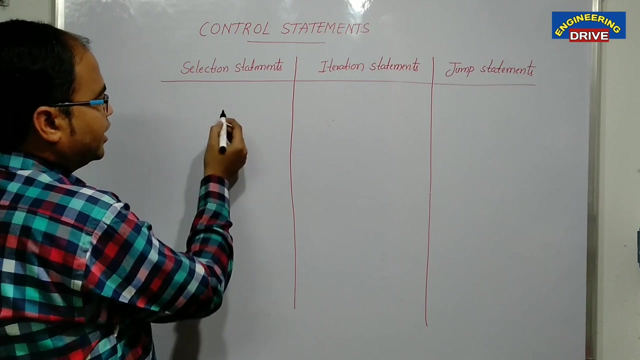 iteration statements and jump statements. what is the purpose of all these three categories of statements? if our program want to shift the execution from one statement to another statement without following a proper order, then we can make use of these three statements, okay, so what is a selection statements and what are the subcategories in this? in our c there are two categories of selection. 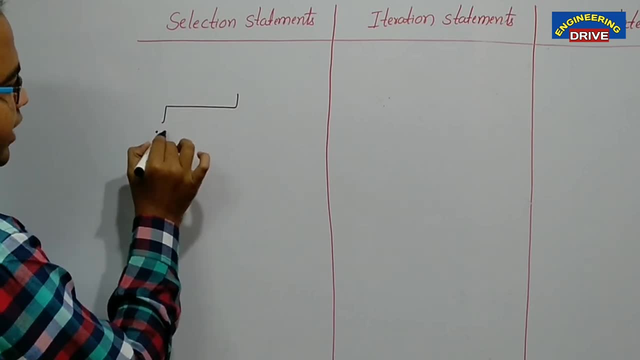 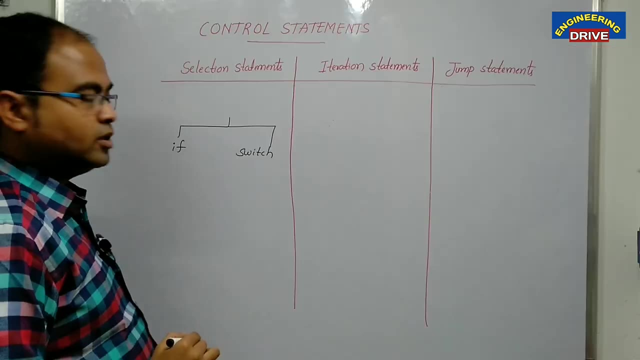 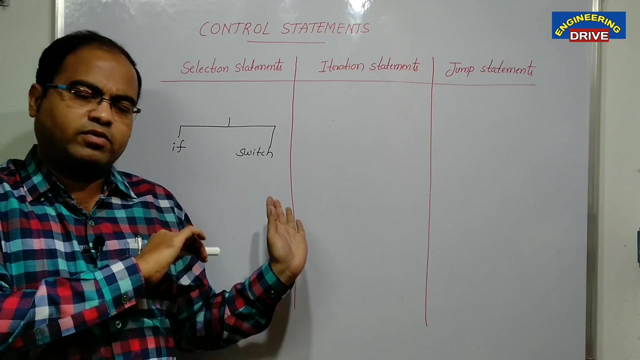 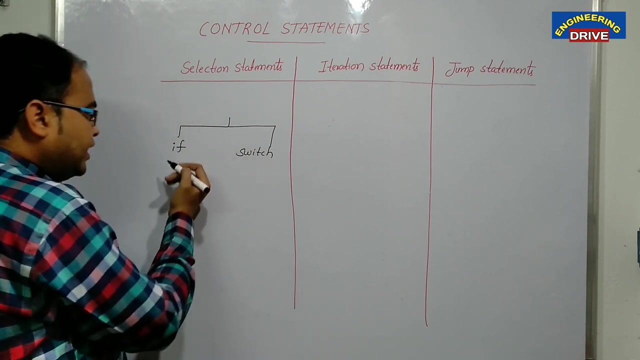 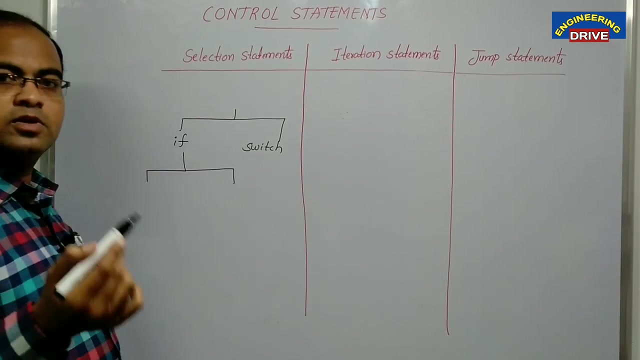 statements. one is known as if, another one is known as switch. so these are the two categories of selection statements: one is a if, another one is a switch. how they will work? what about the syntax? with example program, we will be discussing our next videos. okay, then what are again? this if is classified into four subcategories. so what are those four? 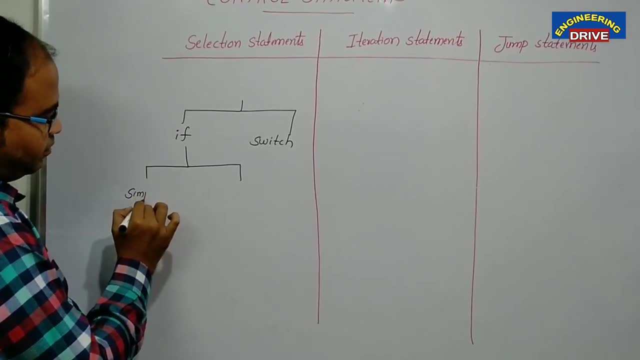 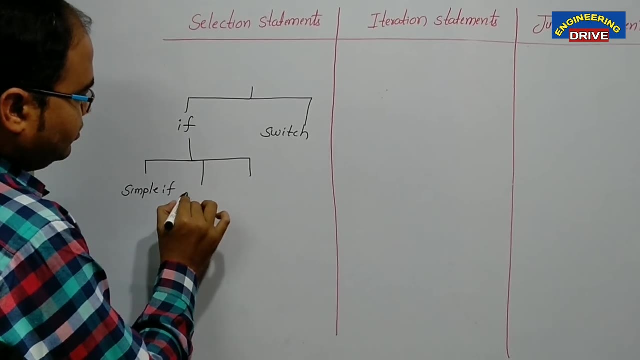 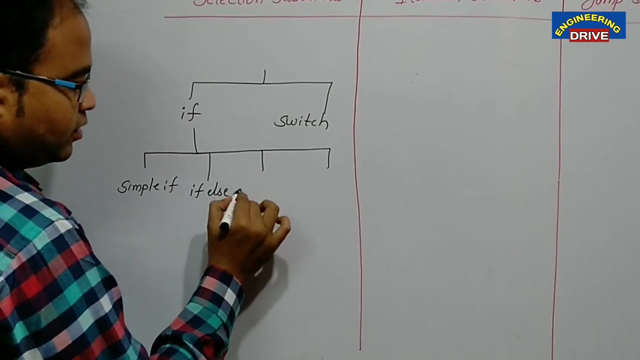 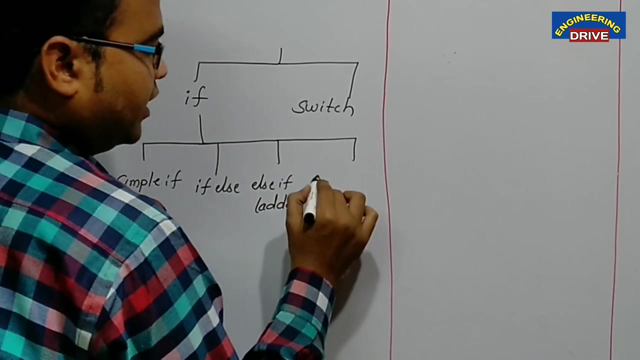 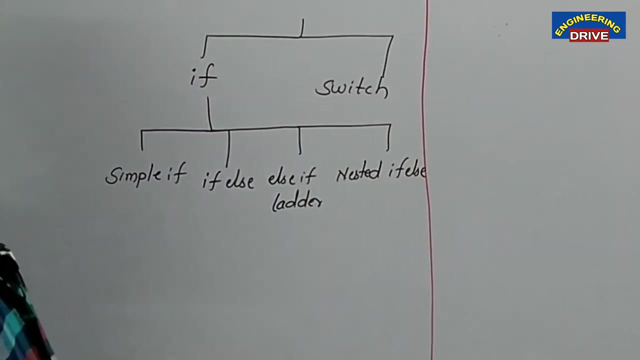 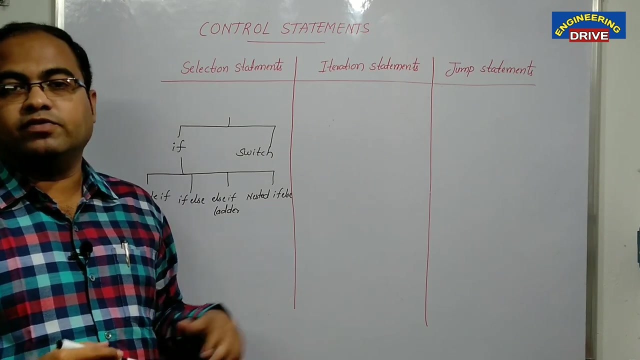 subcategories: simple if. next we are having if, werden last oneies nested if-else? so these are the four subcategories of if: simple if and the most important one is common decentralized standardров. ły simple if and the present final'll y if else lc flatter and nested if else. okay, how they will work when we should select which one. 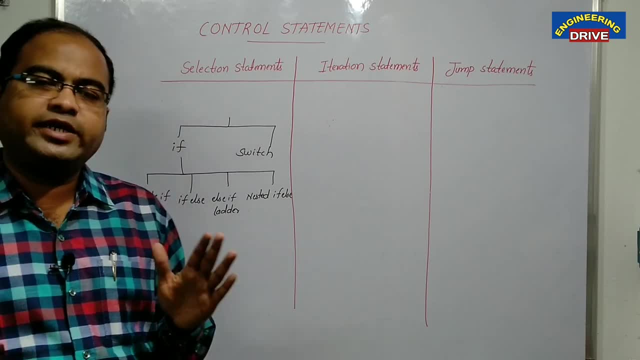 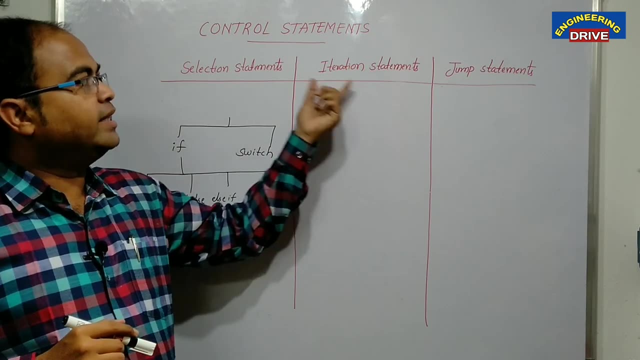 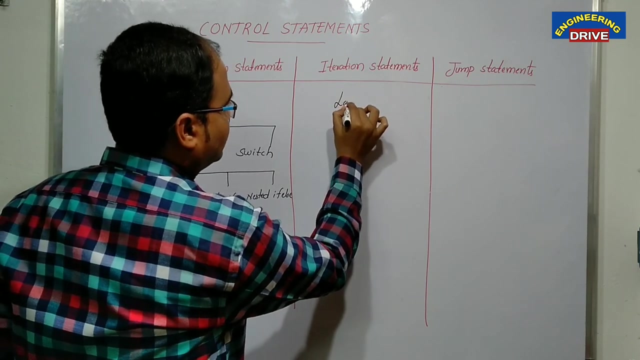 is suitable for us. everything will be discussing in separate video of related to if only that i will be preparing shortly. okay, so these are the two major categories of selection statements and then c- supports iteration statements. also, they are popularly known as loops or iteration statement. if i want to repeat certain part of the program, 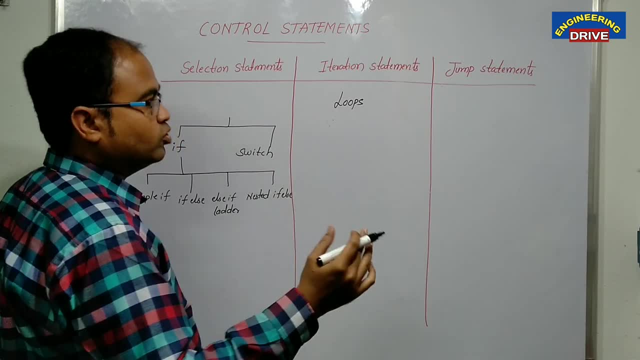 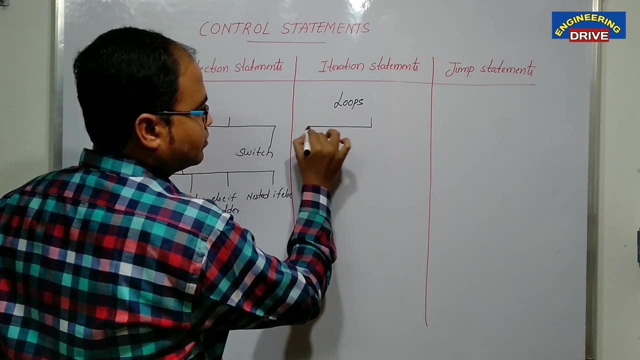 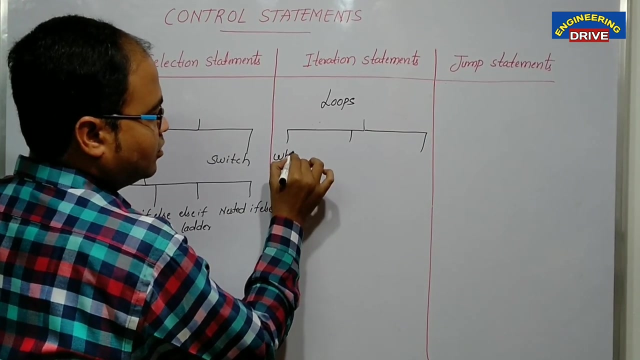 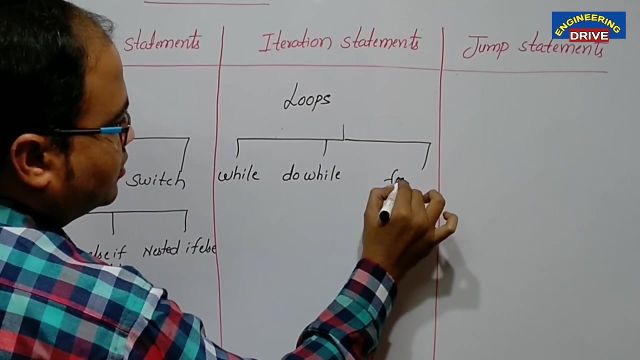 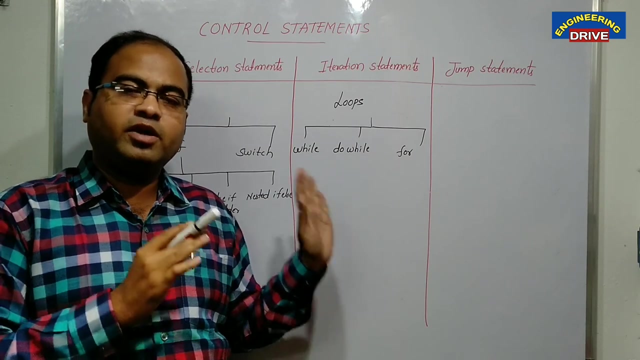 continuously until until certain condition remains true, then i should prefer this: iteration statements. so c language supports three categories of iteration statements. one is while, another one is do while and the last one is for. so these are the three categories of loops or iteration statements. what is the main purpose of using them? if we want to repeat certain part of the program continuously? 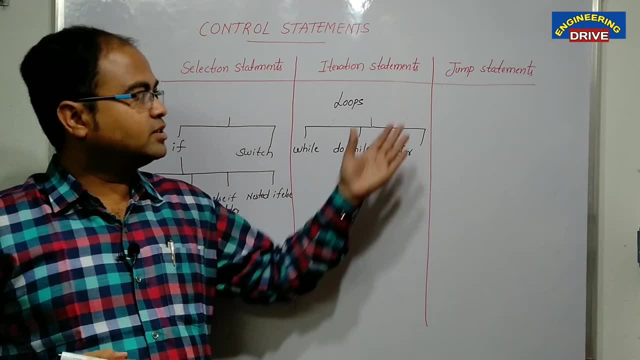 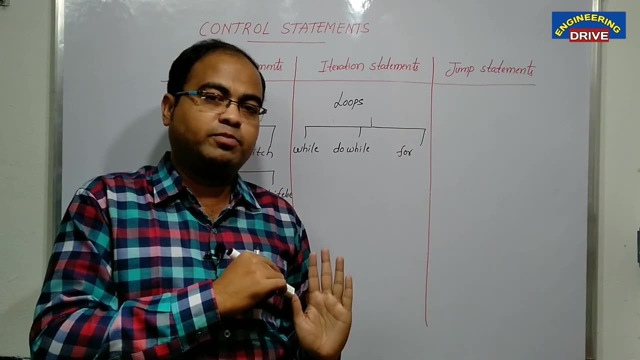 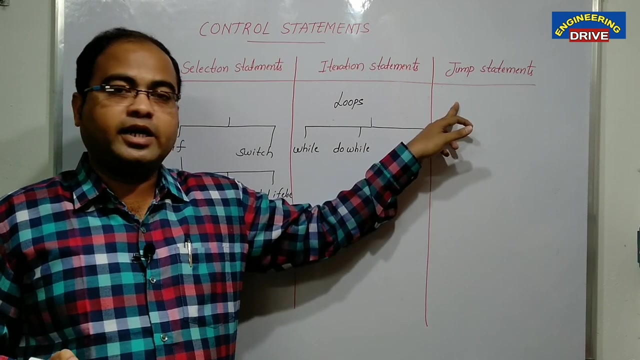 then i can make use of this: loops or iteration statements. and in the name itself. answer is in the third category, jump statements. if i want to make sure that my control in my program will go to some other place where i have specified which i have specified, then i can use this. 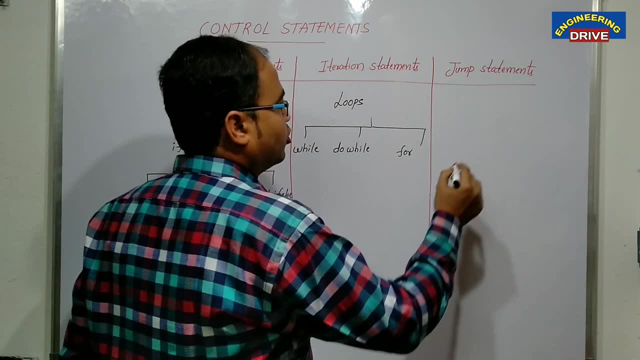 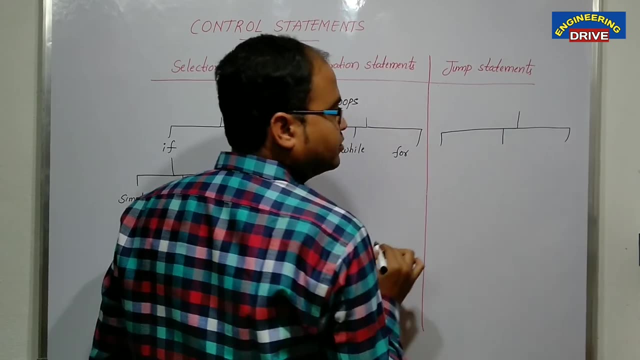 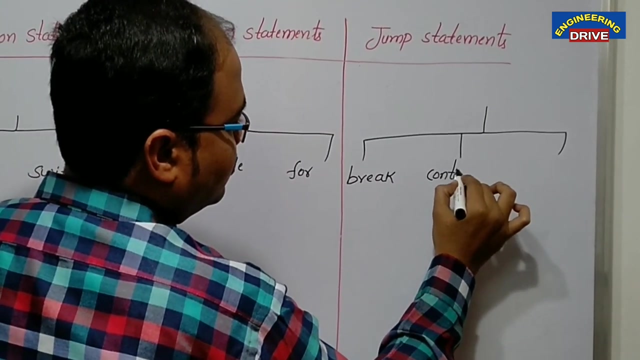 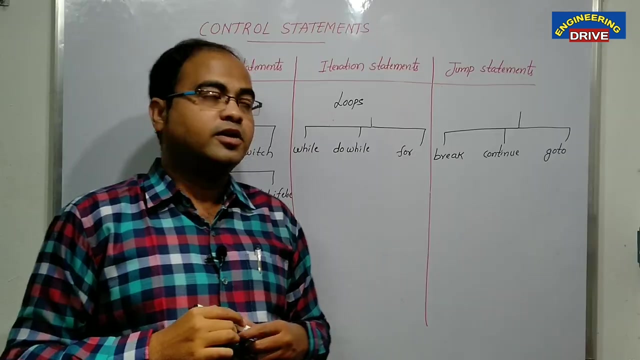 loop or iteration statement, and i can make use of jump statements. so here also, c supports three categories of jump statements: one is break, another one is continue and last one is go to. so these are the different types of jump statement supported by our c language. so, my dear friends, 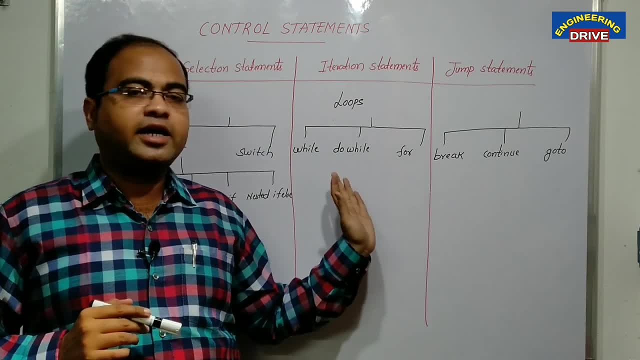 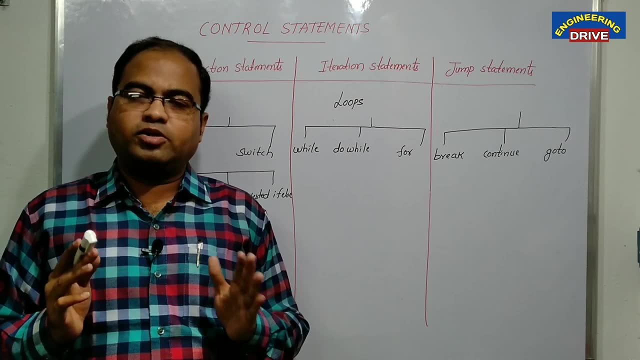 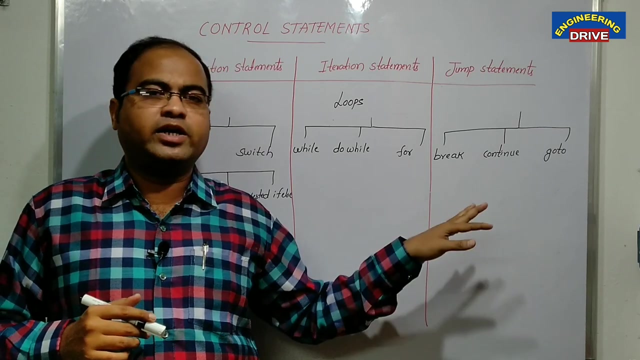 and my dear students, these three categories. if you learn properly, no matter which language it may be, you can able to do your c programs or java programs or c plus plus program very efficiently. i already told you that this topic may be slightly different in other programming languages or there will be. 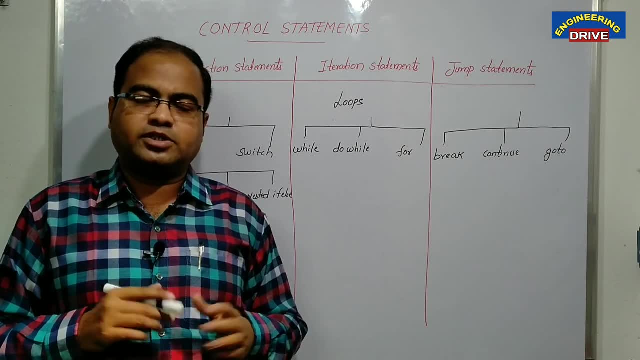 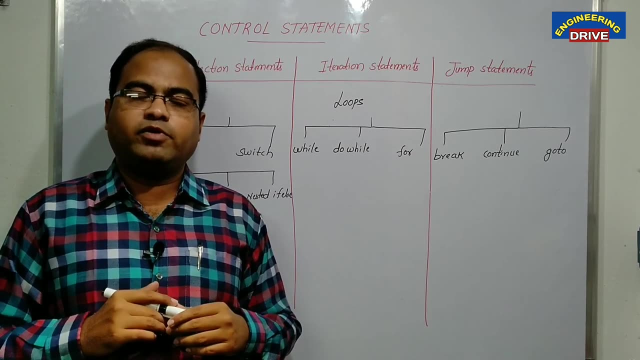 some topics which are excluded in other programming languages. but if you have strong foundation in these three concepts then half of the c programming will be broken down into three and it will become quite easy to you. so you think that the heart of our c language is this. topics: 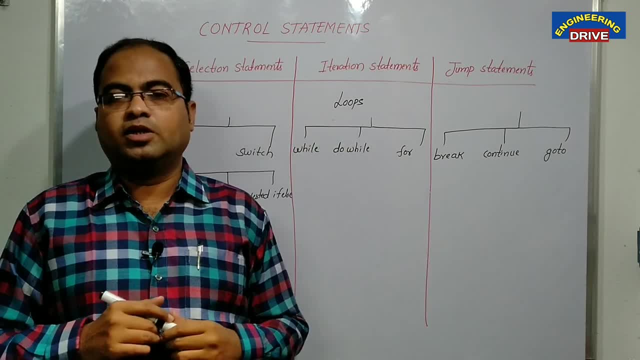 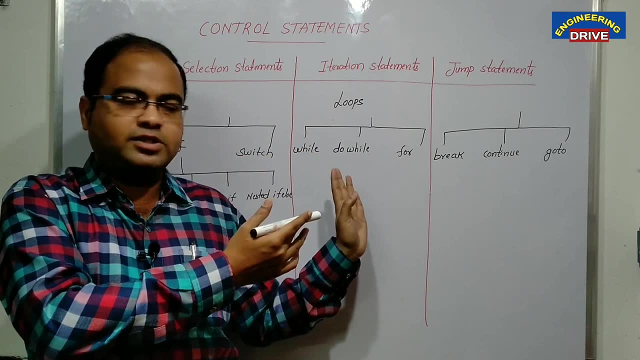 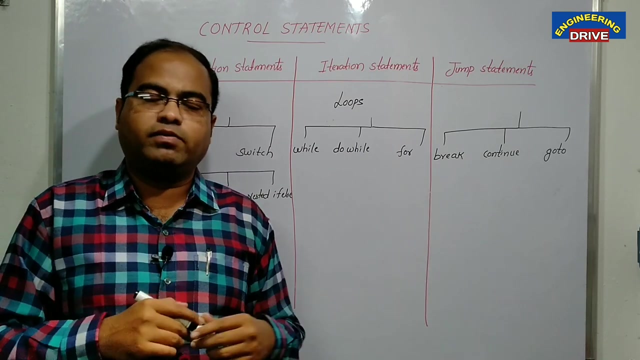 control statements, selection, iteration and jump. so in my next videos i will be preparing separate set of videos for selection statements. if separate video, then switch. separate video then i will be preparing about loops. separate video then i will be preparing about what is how break and continue and go to will work with example programs. main thing is we need to have programs idea. so with